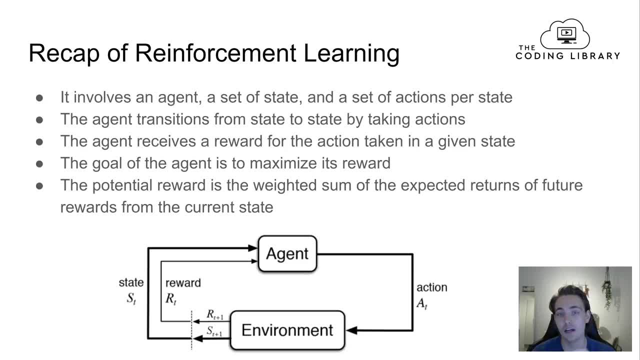 So the agent transitions from state to state by taking those actions that is given or that is available for a given state, And then the agents when it takes actions in the environment, then it receives a reward after that. So we can like give the reward to the agent. 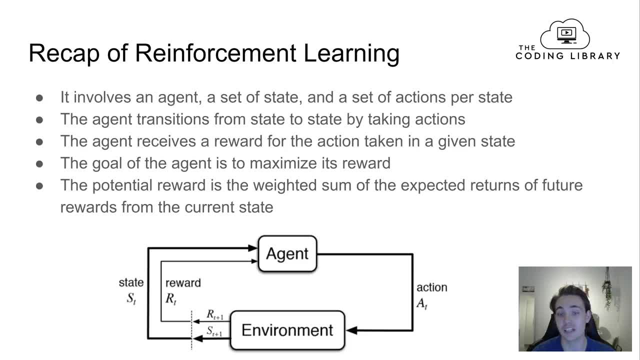 like to like tell it how good it has performed for taking some given action in some given state. So the goal of the agent is to maximize its reward and try to like get the maximum reward by taking all the actions in for any given states to reach its goal and then maximize the reward. 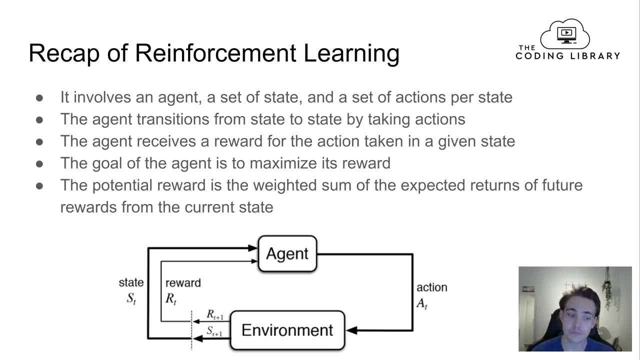 to find like an optimal way to reach that goal. And a potential reward is the weighted sum of the expected returns. So the reward is the sum of the expected returns. So the reward is the sum of the expected returns, of the future rewards from the current state. 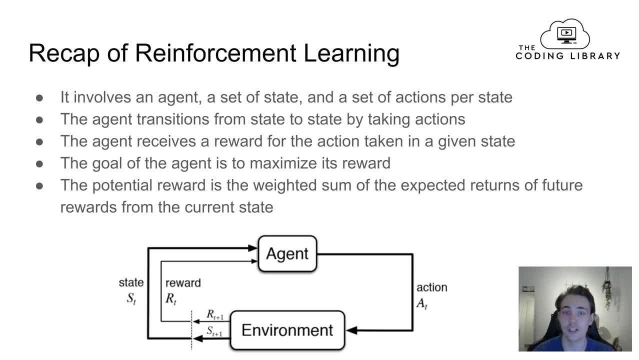 that is currently in now. So this is what we're going to do in Q-Learning And on the next couple of slides here I'm going more in depth with what Q-Learning is and how we can actually like apply this to like get the potential reward. 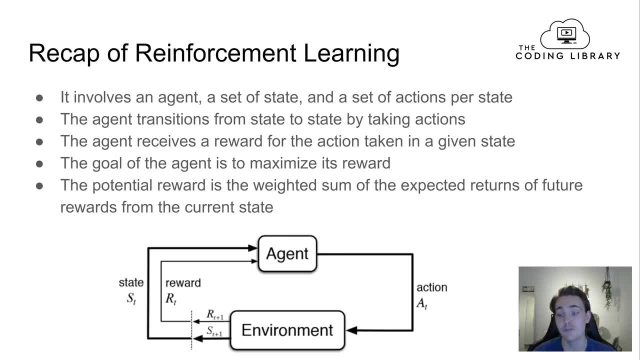 and calculate like the weighted sum of the expected returns of the future rewards from the current state that we're in now and then apply that to find an optimal policy for our agent that it can follow So down. here we have like an example of like how it works with reinforcement learning. 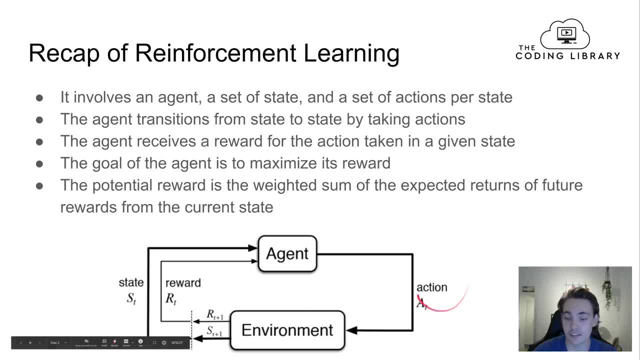 So we have this HTML, we have an agent here that takes some action in the environment at some time. step T here And then for that given state that is in now, it is just the agent is now in a state and then it takes an action in this state here. 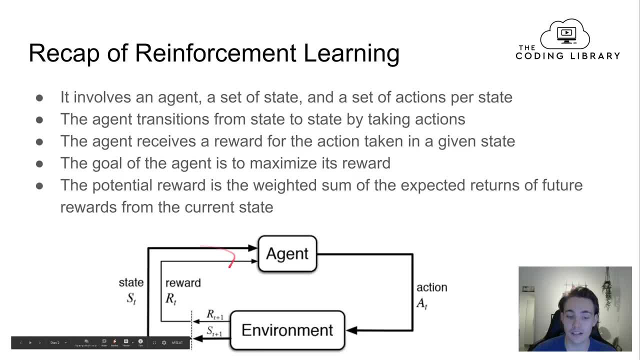 and at the same time step, And then it gets a reward for that action that it takes, for that time step, And then we just go to the next time step. So now we have taken an action and we're transitioned or moved to a new state. 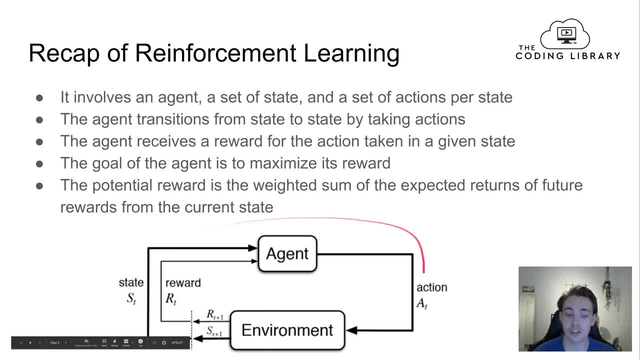 So it will be S T plus one here, And then we just continue doing the same over and over again. So the next state that we're now in is fed to the agent here, And then for that given state it is now taking a new action based on the feature. 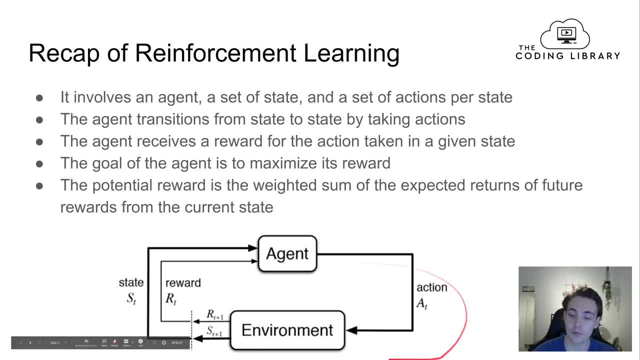 or like the potential rewards in the future, And then we take this action here in environment and we get a new state and get new rewards And it just keeps on doing this And then by doing this, our agent can learn and try to like, calculate. 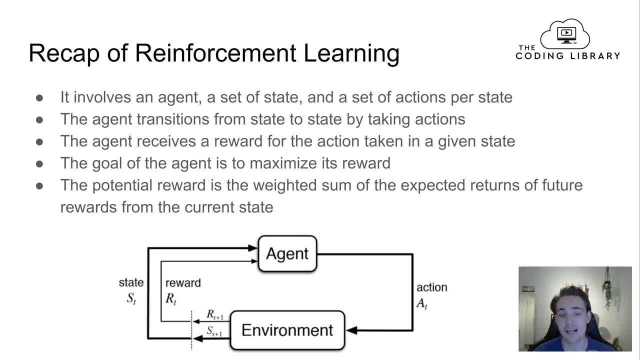 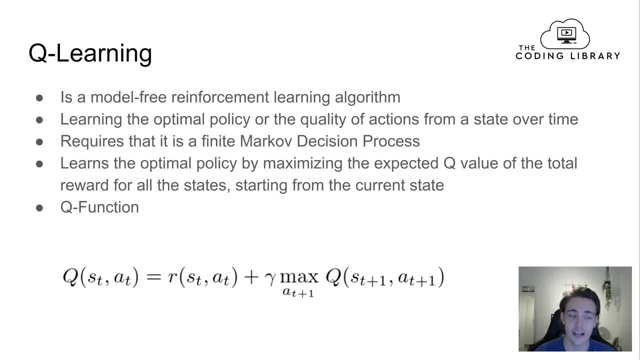 or like try to estimate the maximum reward that it wants to get and then reach the goal in an optimal way. So let's now talk about Q-Learning here, And Q-Learning is a model-free reinforcement learning algorithm, So it means that we don't need our model. 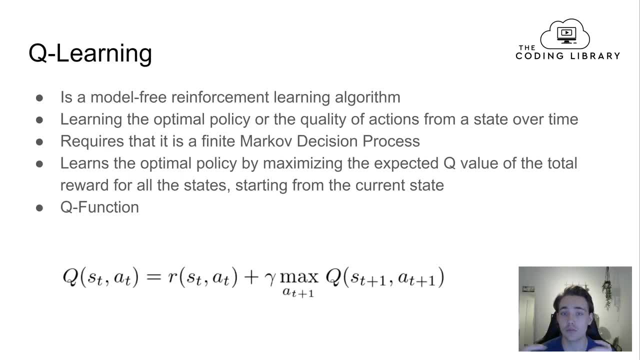 to be fully determined and we can just like place our robot in the environment and then we can have some different kinds of algorithms that either like explores the environment, So we don't need a model when we're dealing with Q-Learning algorithm in reinforcement learning. 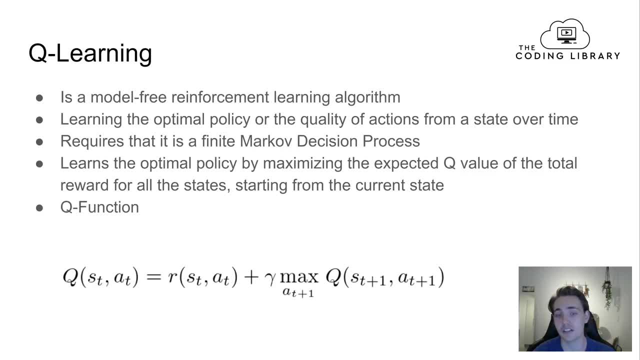 So Q-Learning: it's trying to learn the optimal policy or like the quality of actions from a given state over time. So if we're in a state now, we're trying to figure out what is the best action to take for that state that we're in now. 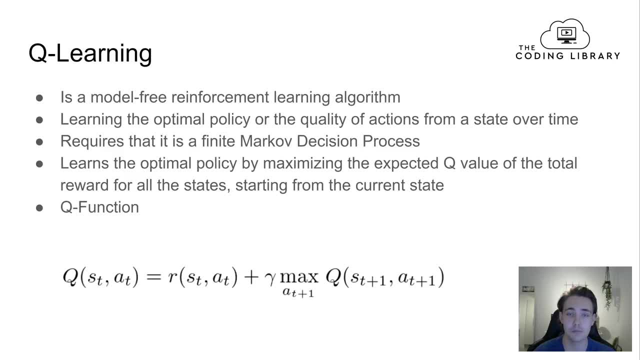 So, then, that is what Q-Learning is trying to find- is the optimal policy that we can just find to get the maximum reward and follow the most optimal path. So we also request that the Q-Learning, or like our process, has this finite market decision process. 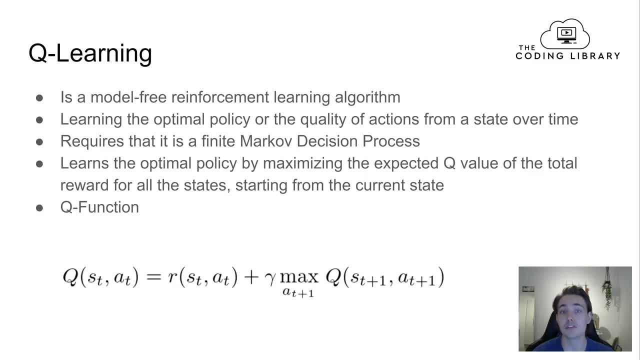 and it has market problems that we have to implement in order to get the maximum reward. So the action that we're taking now is only depending on the state that we're in now and not on the previous states that we've been in. So it's only the state we're in now. 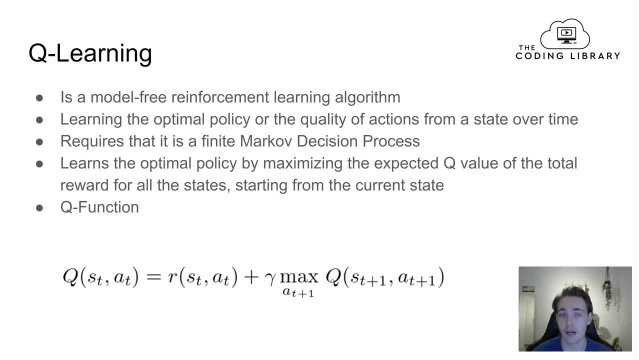 that we're taking action from And if we want some information from the previous states like we have to implement it in the given state by using some memory. So Q-Learning: it learns the optimal policy by maximizing the expected Q-value of the total reward for all the states. 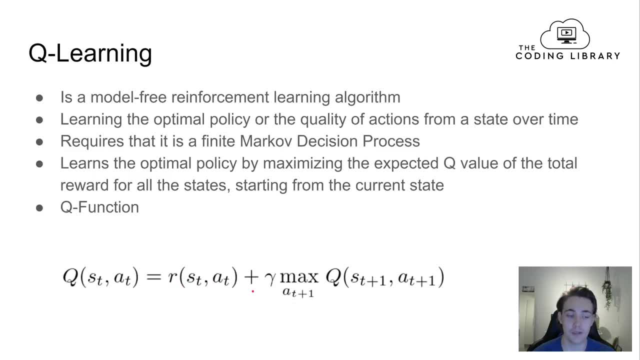 starting from the current state that we're in now. So this is like what we can set up here down in the Q-Learning which we're going to apply when we're going to apply a Q-Learning in code. So we have this Q-value here for a given state. 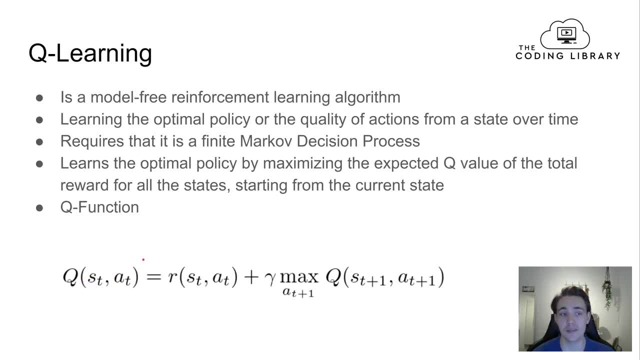 and an action that we take. So this is like the Q-values here that we're going to update our Q-table with in Q-Learning And then that state here or like that value- this Q-value here is equal to the reward for this given state and this action that we're taking. 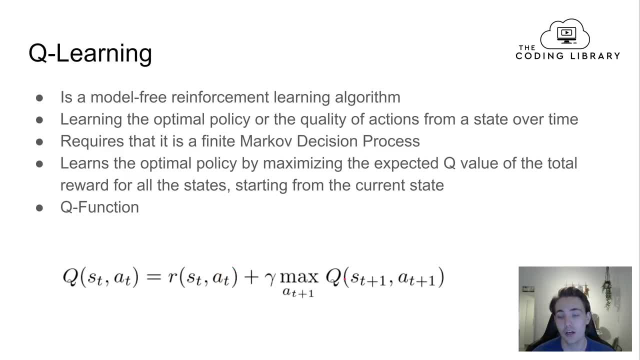 plus the maximum rewards for all the other states and state and action pairs for that given state we're in now and the action that we're taking, And then we can scale it with some kind of factor here if we want to have our other rewards having more impact or less impact. 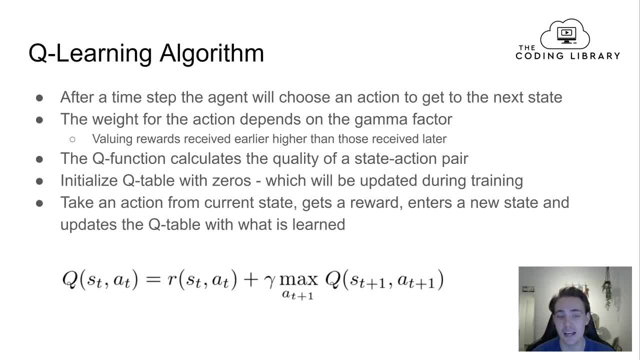 So the Q-Learning algorithm. here it's like after times that the agent will choose an action to get to the next state. So we're in a state now and we're feeding that state to our agent and then it will take some action. 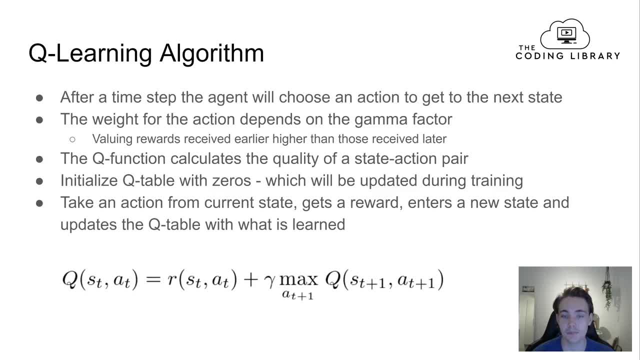 in this state now, And then the weight for the action depends on the gamma factor, as I just talked about, So valuing the rewards received earlier higher than those received later. So we can just then scale like all the values or all the rewards in the future. 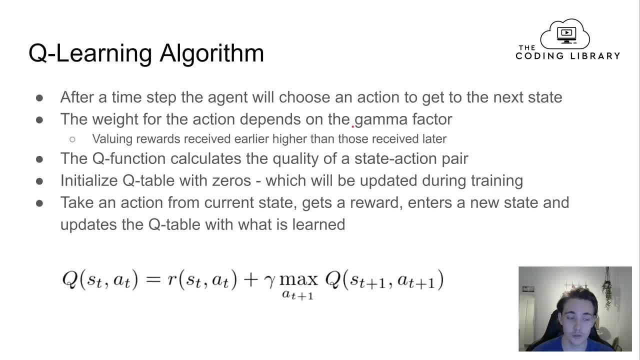 with this gamma factor here which we're also going to use in Q-Learning in the example that we have in the code. So the Q-Learning function here: it calculates the quality of a state-to-action pair, So it tries to measure how good. 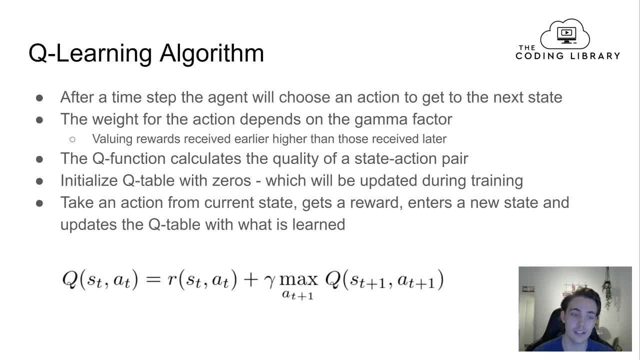 an action is for this given state that we're in now, And then we will have this Q-Value here that we're updating our Q-Table with. So first of all, with this Q-Learning algorithm here, we have to initialize our Q-Table with zeros. 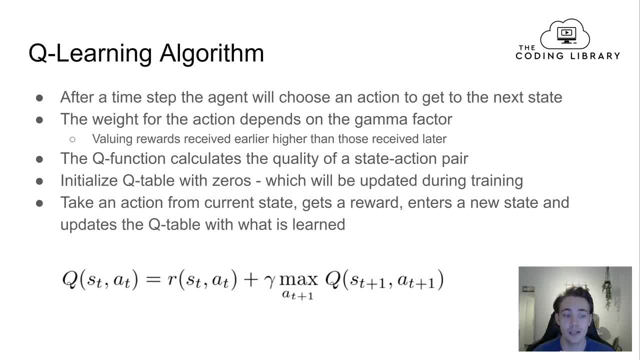 which will be updated during training. We can also initialize our Q-Table with nothing and then update our Q-Table when we're visiting a new state, for example, So we don't have to like initialize a big Q-Table if you have a lot of different kinds of states. 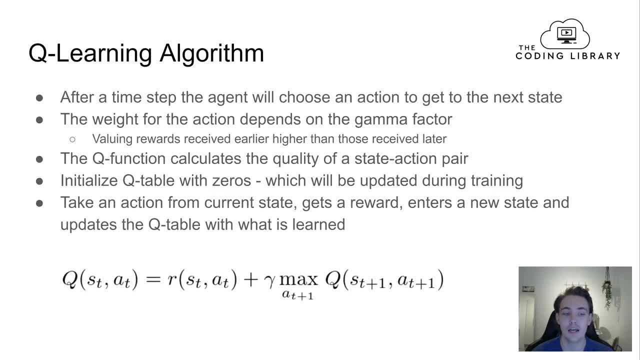 Then we can just have our agent exploring the environment and then and then update the Q-Table and then insert the states that we're visiting while exploring the environment And then, when we have done this here, we have taken an action from the current state that we're in. 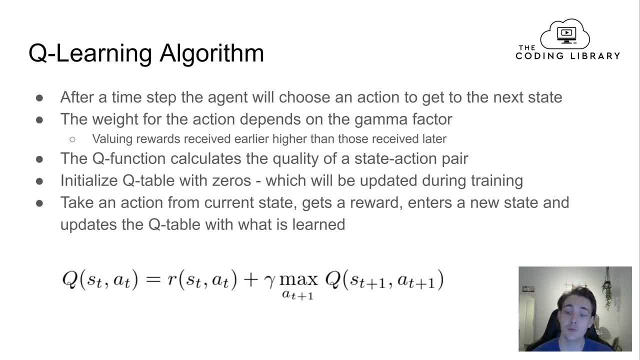 We get a reward for that action we've taken And then we enter a new state with that action and then we update the Q-Table with what we have learned and with the reward that we have that we were given for taking that action in that state we were in. 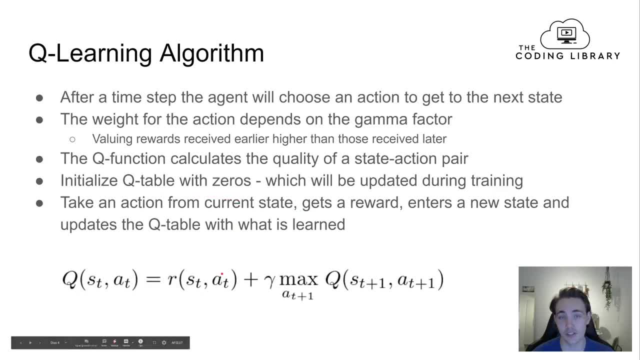 So this is what this equation, or like this function down here it says, And this is what we're going to actually like imply in code to apply this Q-Learning algorithm. So this is the example that we're going to use and we're going to implement in code. 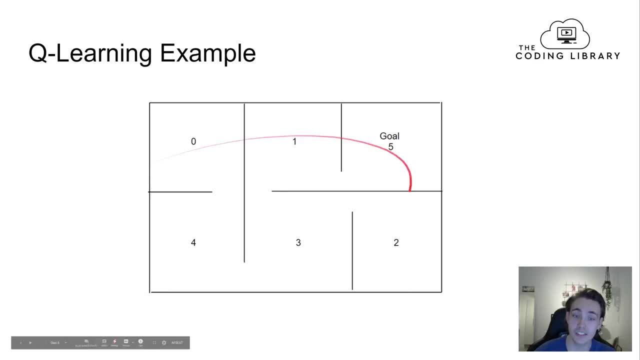 So we have this Q-Learning method here, or like this example here, where we have these different kinds of rooms here, And then we're going to initialize our agent in a random room here from one to four or for similar to four, And then we have this fifth room up here. 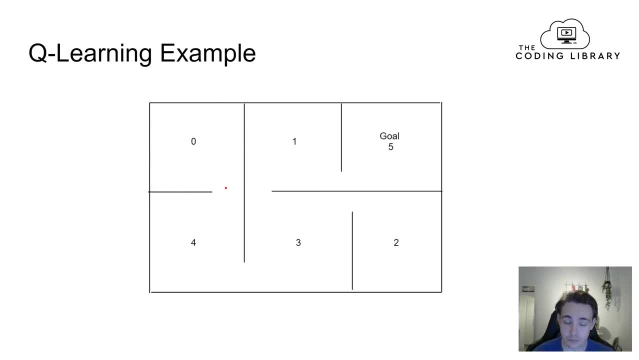 which is the goal room that we want to reach. So our agent will be put in one of these rooms here and then it will try to figure out how to get from that room that it's placed in to the end goal here five, And then it can also like, for example, 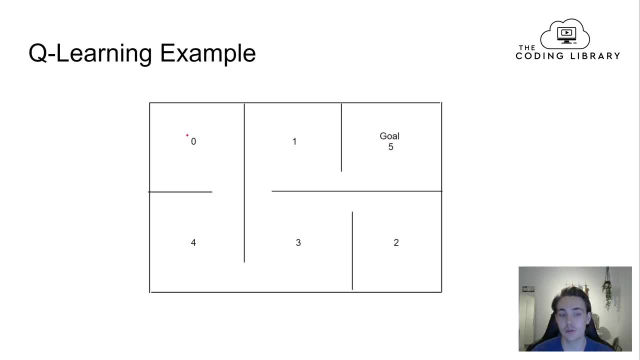 from the second room, the Seraph room- here it can only go to room four, And then from room four we can go to three and one and then to five. So that will be a valid path for the agent to take in this environment here. 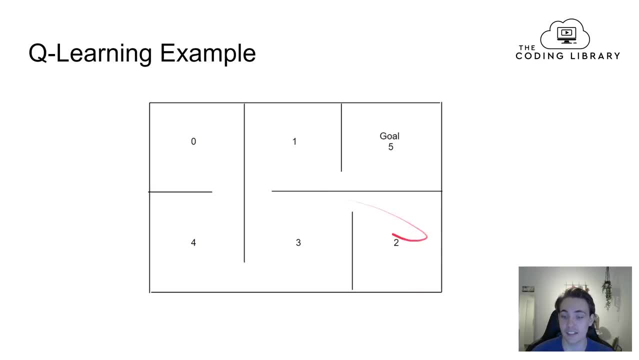 when it's trying to figure out how to get to the end goal. And if we were in the second room here, we have to go from two to three to one to five. So this is the example that we're going to apply and implement in code. 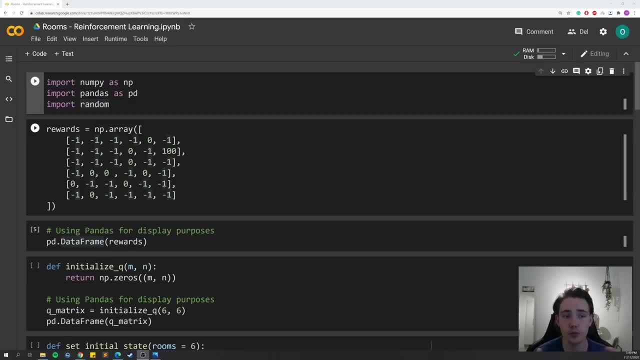 So we're going to go up here and this is like the kind of ID that we're going to use to implement this queue learning algorithm here. So, first of all, we're going to impart numpy, pandas and random, because these are the modules that we're going to use. 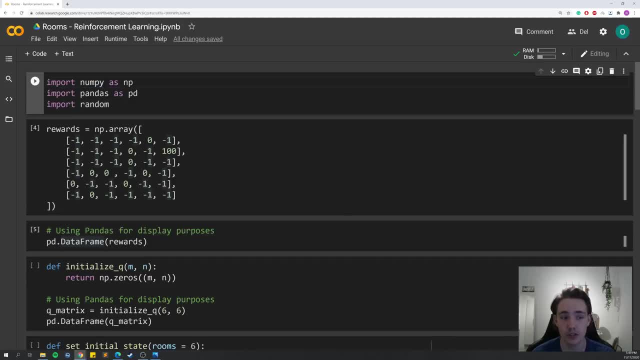 to like create the queue table and also the reward matrix, and then pandas to show the data frame and get like a more intuitive way to see what's going on. And then the random module: here because we need to initialize our first state or our initial state as a random room. 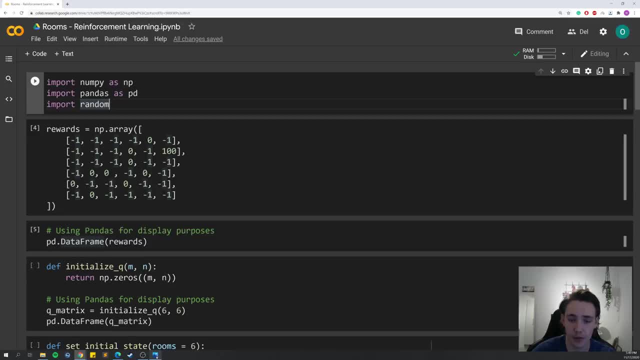 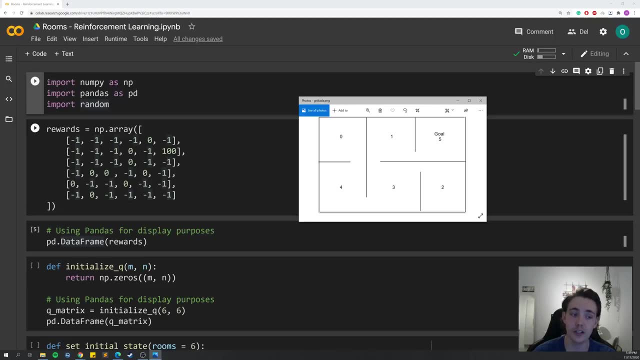 Then, first of all, we have this reward matrix here that we're going to set up with the environment, So we know that we have the different kinds of rooms here, and then we set up the rewards for all the rooms here. So on the rows here. 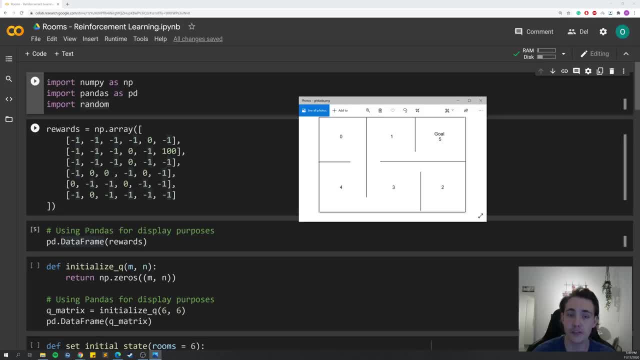 we have the rooms and then on the columns we have the actions that we can take by being in some state or in some room. So in this case, here we have minus one if we don't have a value or a valid path, or like a valid trajectory. 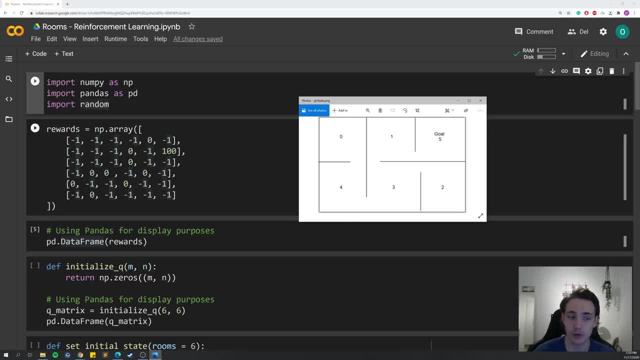 between one of the rooms and we will have a zero. if we can, for example, go from room zero here to room four, then the action four here will have a reward of zero, because we're able to go from room zero to four but we're not able to go from zero. 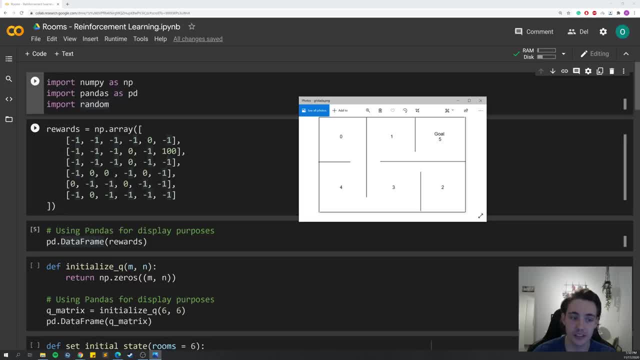 to any other room than four in this case. So in the case here of the first room, we know that we can go to either goal three, which is this zero here, or we can go to the end goal here, which will return a reward of 100. 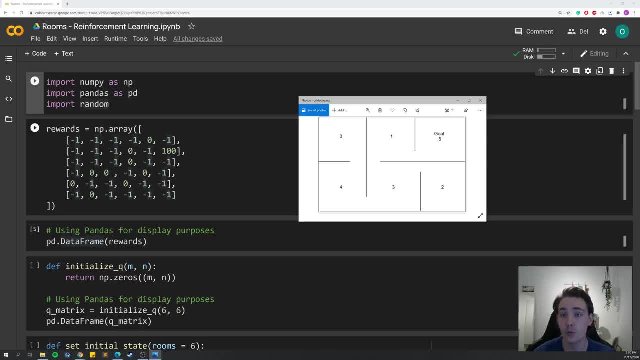 because we want a really hard reward when we reach this end goal for our agent. So it will be able to learn that reaching this fifth room here, or room five, is really good, So it will like get a really huge reward for getting to this end goal here. 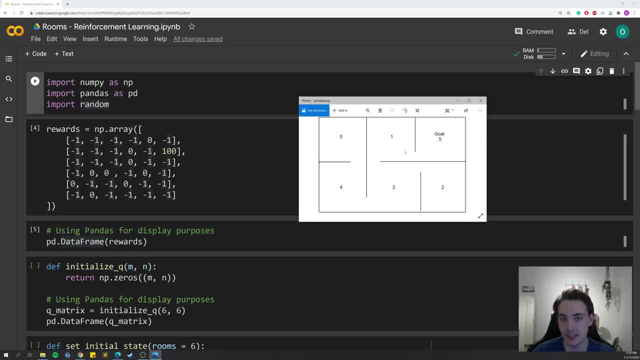 And we can only get to end goal by being in room one here. So this is what we set up in our reward matrix here, which is kind of like in the environment that our agent is going to operate in. So we've just run these cells here. 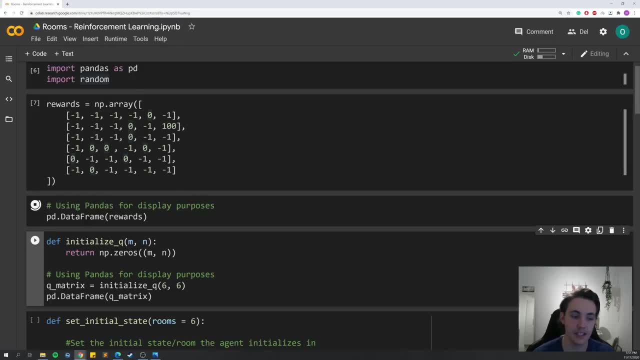 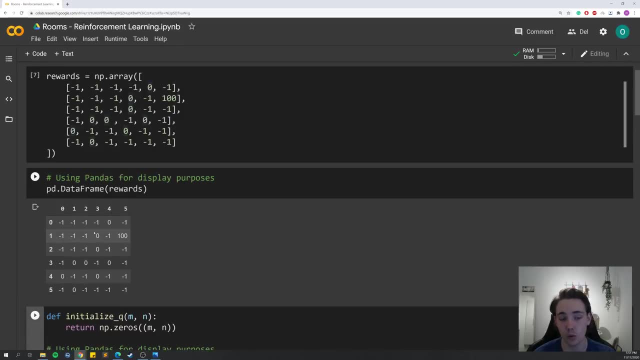 We use the Pandas DataFrame here to visualize it better. So we have this environment matrix, or our reward matrix, which is yielding the rewards that our agent can get for some given state and some given action that it takes in that state. So we have the rooms down here. 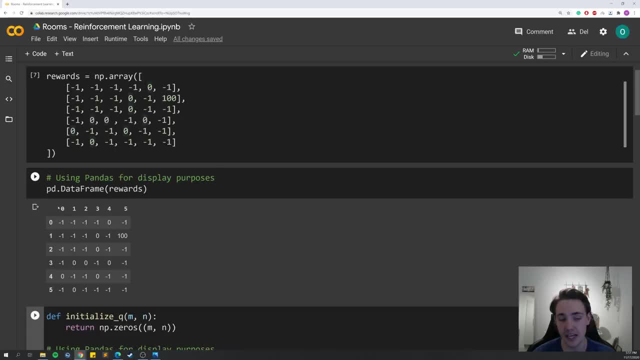 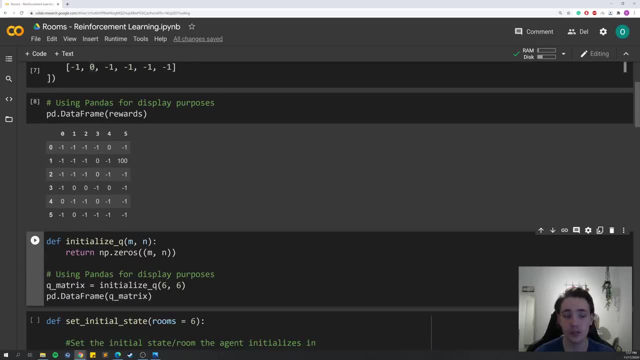 on the rows, and then we have the columns here, which is the actions that we can take for some given state. Then, first of all, we have a function here that can initialize our queue table with zeros. So, in this case, here we're just going to hit this here. 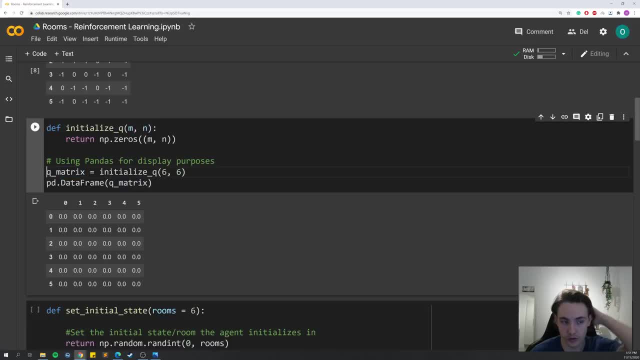 We have this queue matrix here that we're going to initialize with a six by six grid here- six by six grid- And then we will initialize our queue table here, which we're going to update when we're learning and training with our agent in the environment. 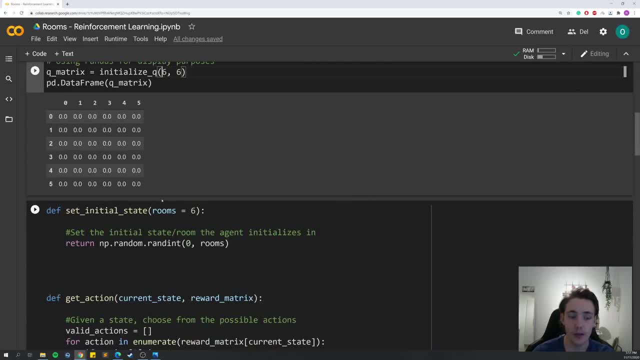 Then we have a function here to set the initial state. because we want to get a random initial state, So we have this room here as default, so the rooms here will be six as default, And then we just return a random number between zero and six. 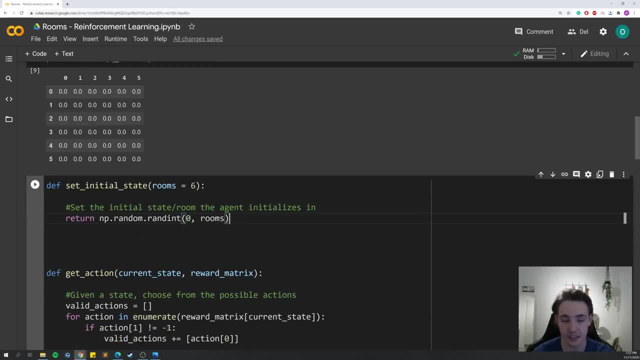 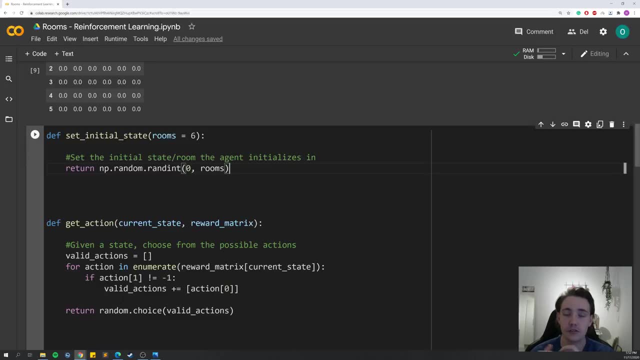 which is the rooms that we're going to initialize in or, like, set the initial state to. Then we have a function here to get the action that we're going to take for some given state. So to take some action in some given state, we need to know the current state. 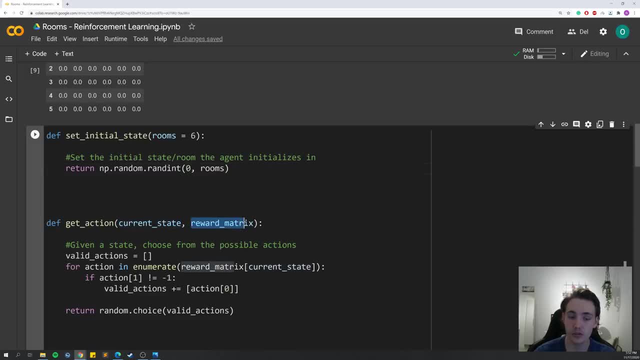 So we'll pass that as parameter And we also need to know the report matrix so we can go in and see what different kind of actions can we take in some current state that we're in. Then we have a new array here that we have the valid actions. 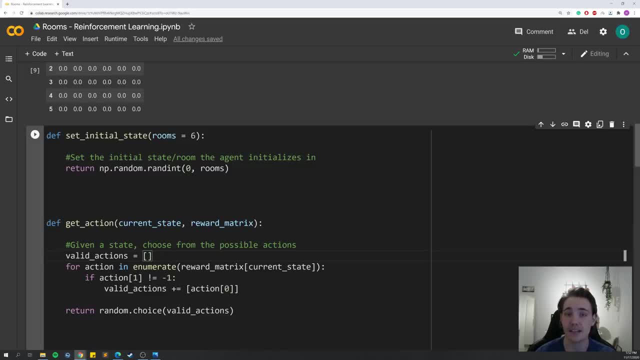 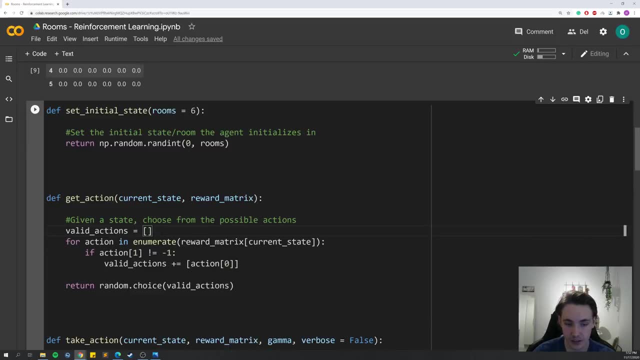 that we can take, because we can only take an action if we can actually go to the other room, to another room or to go to the end goal. So then we run through all like actions here in this report. matrix here for the current state. 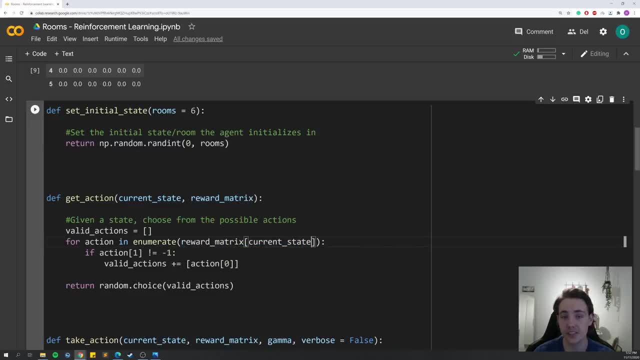 So we run through all the actions in our current state that we're in And then we see that then we say that if the action is equal to minus one then it's not a valid action. So if it's not equal to minus one here. 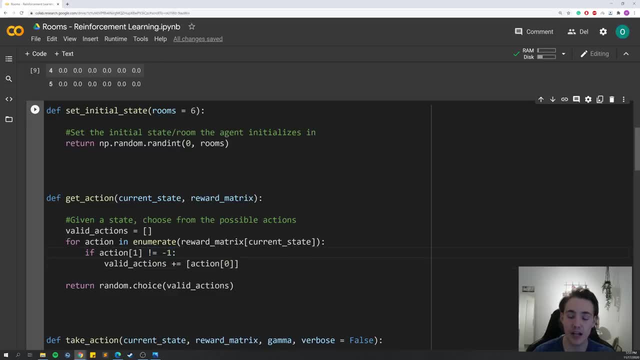 it will be a valid action, And we just add that action here to the valid actions. So after that we can then take a random choice of the valid actions here, because we haven't learned anything yet, So we don't know which action is best to take. 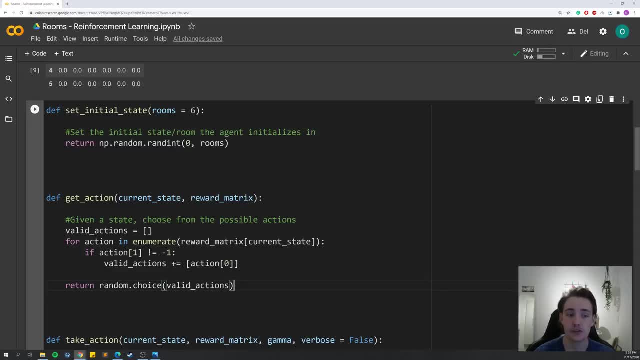 So when we're learning here, we're just going to take a random choice when we get the action here for the first time for some current state here, because we don't know what is the best action yet, So we're just going to take. 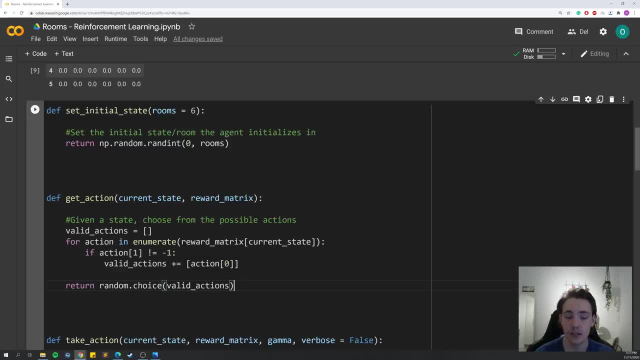 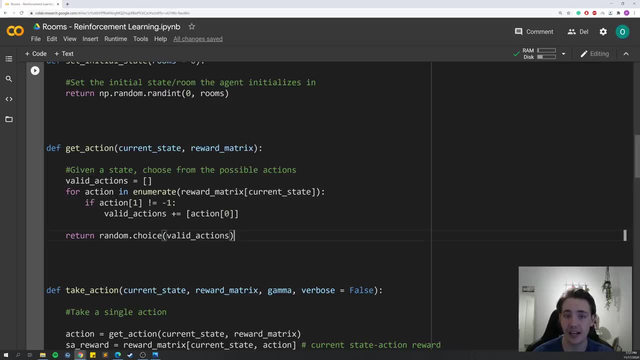 a random choice. when we get the action here for the first time because we haven't learned anything, And then when we have this get action function here, we can actually like return an action for some current state by using this reward matrix that we have set up. 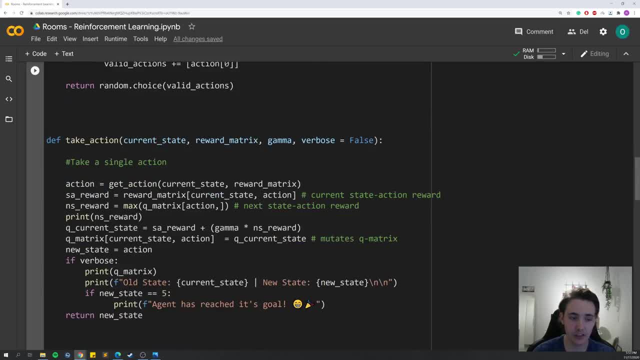 for our environment. And then we have a function here which is like, kind of when we're going to implement the Q learning function that I showed you in the slides as well. So we have this function here to take an action and we need to pass. 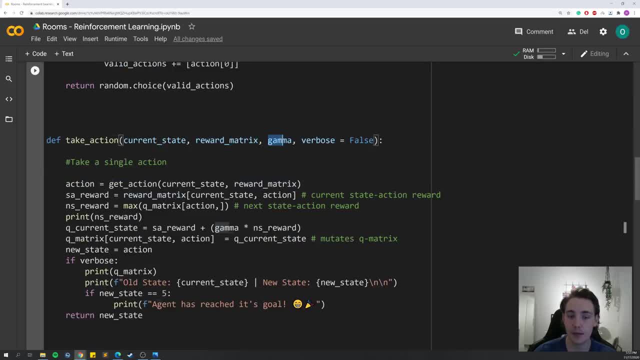 the current state that we're in the reward matrix, and then the gamma, which is the scaling factor of the future function and the future rewards, And then we have this rows here if we want to display the output. So first of all we have to take 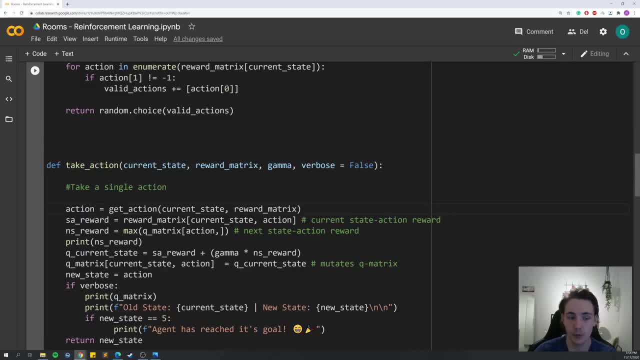 and we have to get an action here by using this function that we just talked about, which is to get action here for some current state and the reward. So now we have taken an action here and we have this action stored in this variable And then we will calculate. 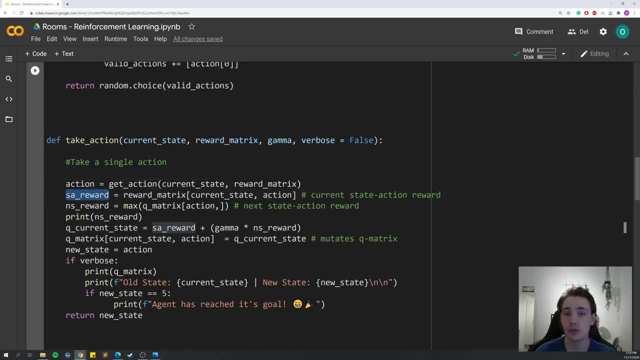 like the first part of the Q learning function, which is the current state action reward, And then the reward will be like this reward matrix here for the current state and then the action that we chose to take in this current state that we're in. 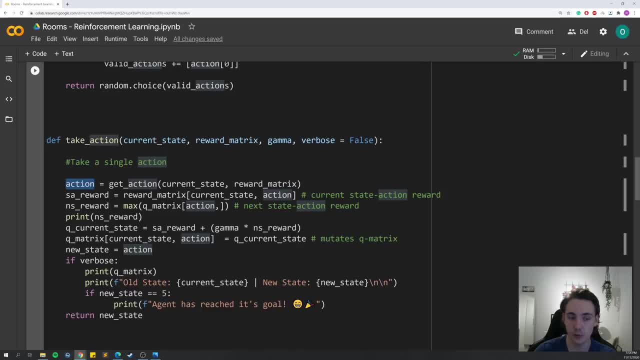 So this is the added reward that we get for taking this action here with this get action function here, And then we have the second part here, which is the future rewards for the actions to take and to get to the next state, which is the next. 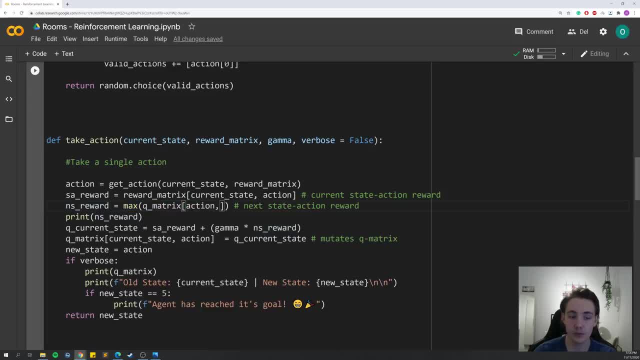 state action reward. So we take the maximum value of all the states that we can get to by using this action here, in this Q matrix here, And then we have the Q matrix. So in this case here our Q matrix is zero for the first time here. 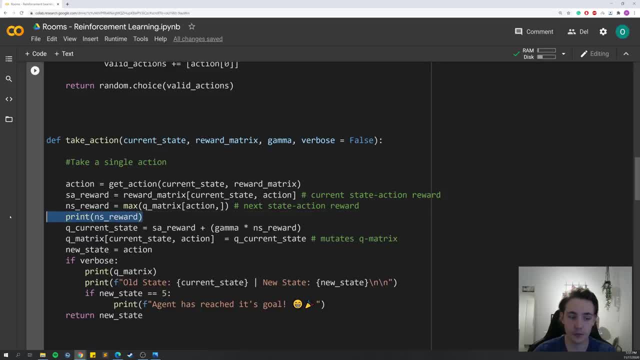 but it will learn over time And then we just print out the reward- here We don't need to do that- And then we can set that the current state value here for our Q function will be this value here, the first part that we calculated. 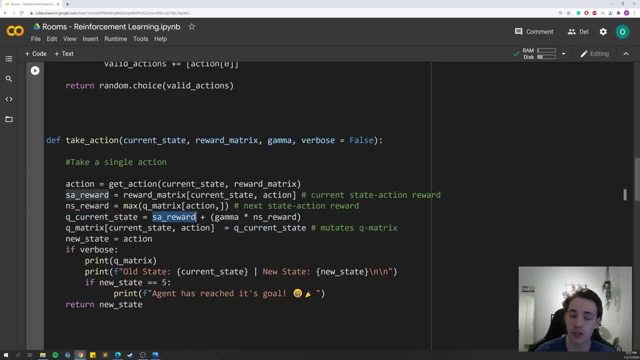 plus the gamma factor, which is the scalar to this future reward, And then we multiply that with the NS reward here. So this is exactly the function, like these three lines. that we're doing here is exactly the same that we're doing for the future reward. 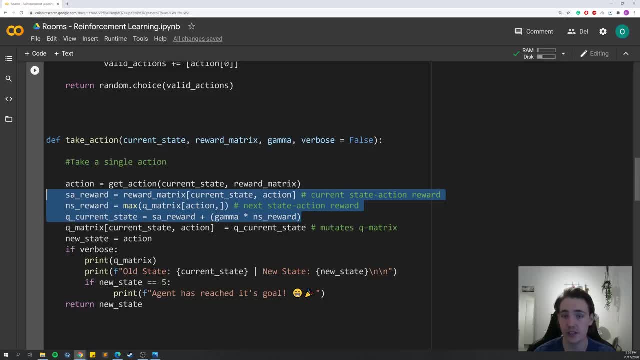 And then we multiply that with the NS reward here. So this is exactly the same that we're doing here is exactly the function that I showed you in the slides with the Q learning and the Q function, And then we can say that we can then. 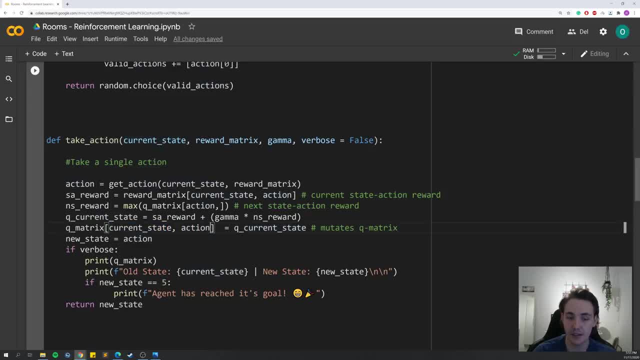 now update our Q matrix here for the state that we're in and the action that we're taking, And then we can set that equal to this Q value that we calculated with this function up here. So now we're updating our Q matrix and then it will update. 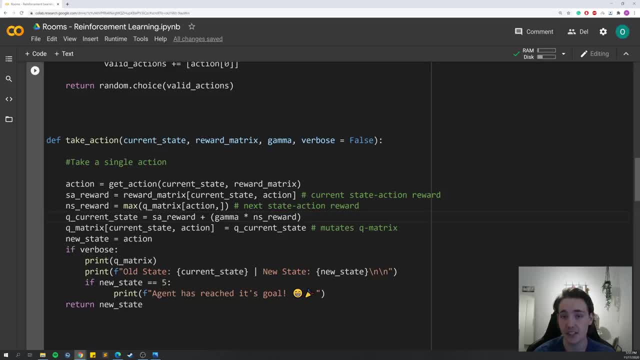 over time and try to estimate the reward matrix that we initialized in the start and trying to figure out what is the best path to get to the end goal. So now we set the action that we're taking to the new state, because when we our action, 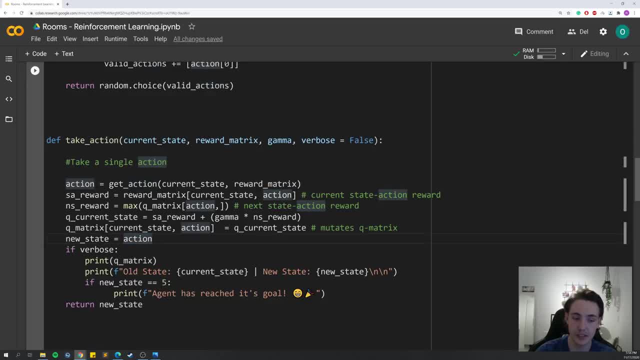 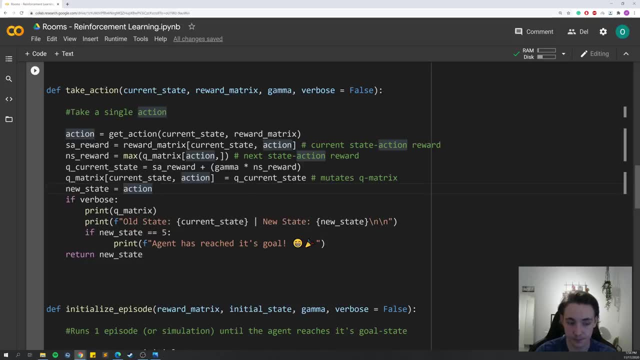 when we take an action, we will now transition to a new state. So we set the new state here equal to the action, And then, if we want to print it out, it will just print out the matrix here and it will print out the first state here. 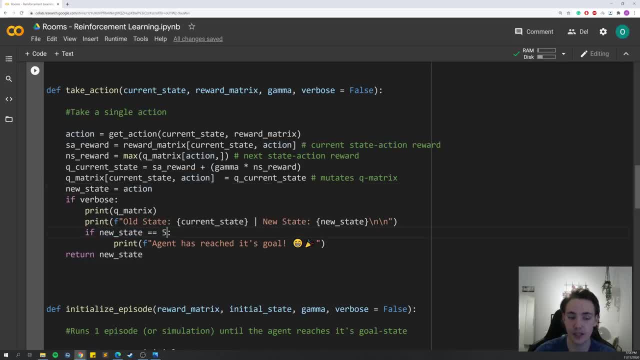 And if we're in state five, we just print out that the agent has reached its goal and we can now terminate our episode when we're going to train, And then we return the new state here for this action. so we know that we take an action. 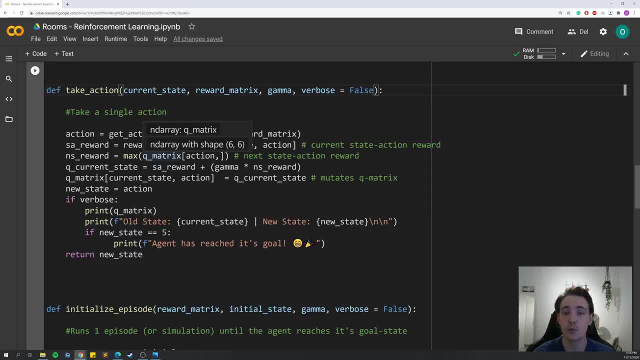 and then we calculate the reward for that action we take, We update the cue table and then we return the new state that we're in by taking this action in the environment with our agent. Then we can go down here and initialize an episode. so this will be. 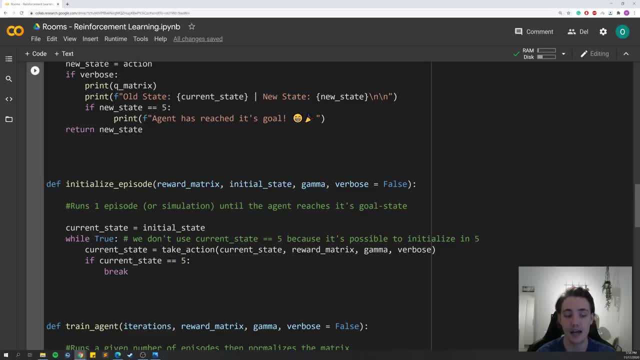 like the first episode, and then we can have when we're training. we're going to initialize this multiple times, so we're going to train and call this function like multiple times to update our cue table. So first of all, here we have, like this current state here: 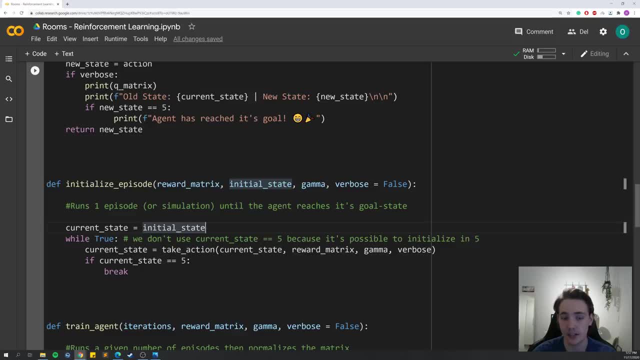 is equal to the initial state, and this initial state here will be a random initial state for every time we train our model or every time we call this initial episode function here, And then we're going to run while through here, and then it will just run. 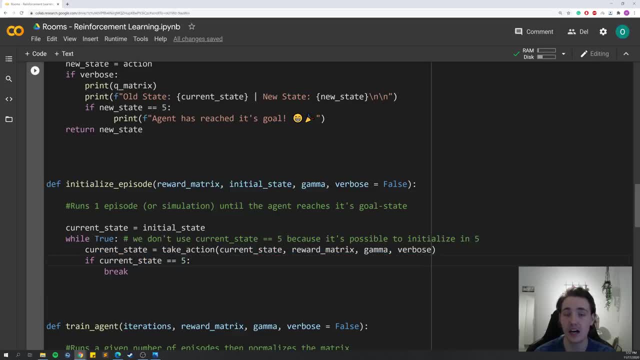 until, like, we are at state five, which is the room five, and we have reached our goal, and then we just have this current state here, which is equal to the action taking. so we just keep on taking action and then we store it in this current state here. 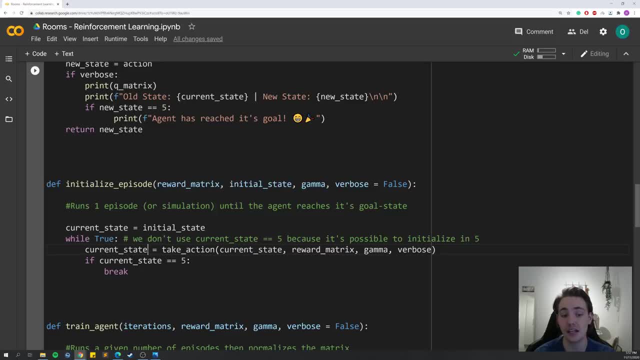 and when we take an action that is equal to five, that results in new state equal to five, then we know that we have reached room five and our end goal and we can then break out here and our episode has finished and we have updated the cue table. 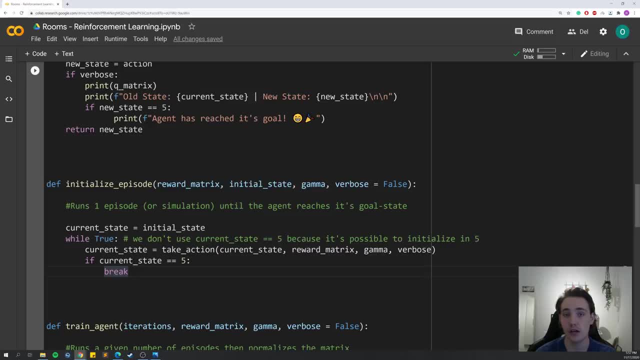 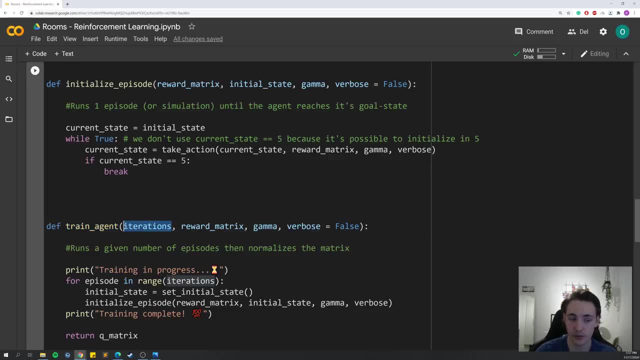 So this is how to run one episode of our training process. So to run this multiple times, we have this train agent function down here which takes like the number of iterations or like the number of times we want to train our agent and it takes the reward matrix here. 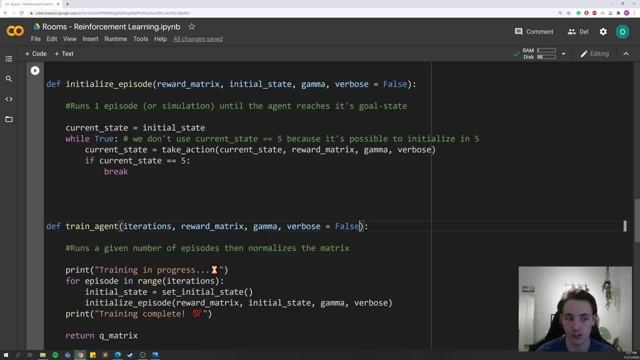 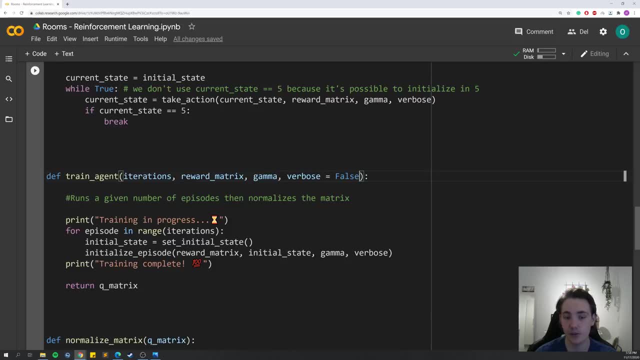 the gamma scaling factor here and if you want to display what's going on. So when we have this train agent here, it runs a given number of episodes and then normalizes the matrix so we can see the result. So first of all, we just have a follow here. 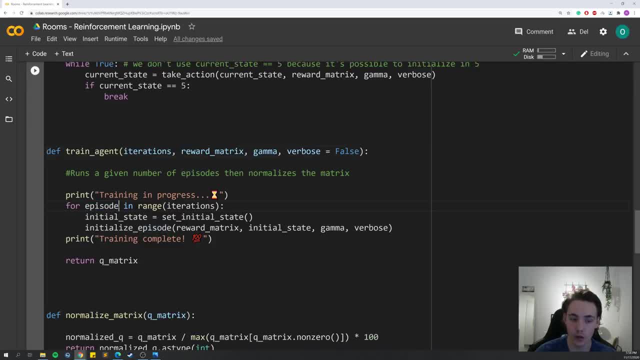 that has one episode here. so we run through like one to the number of iterations or like the number of episodes that we want to train our agent on, and then we have this initial state here, which is just set, equal to set initial state and the initial state here. 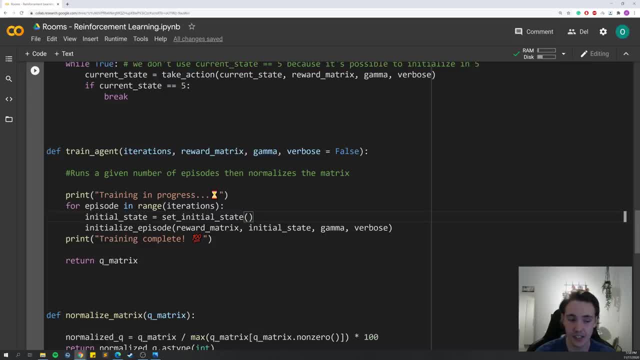 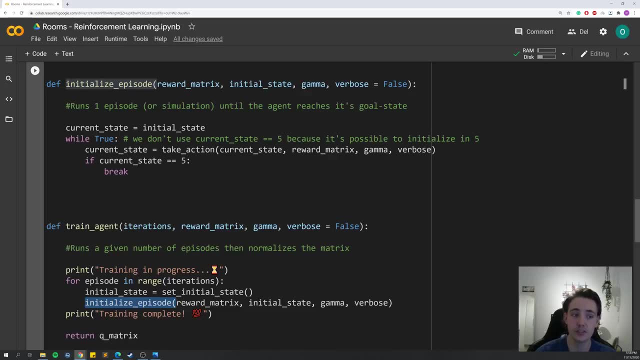 is just a random initial state, and then we have this initial episode here, which we just talked about is the kind of is the function that we're going to run over and over again. So this function here is one episode and it will terminate when our agent 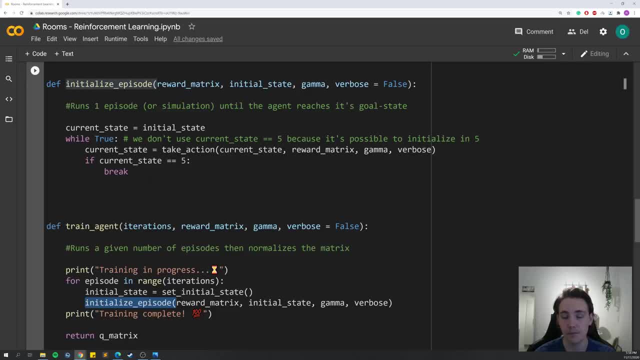 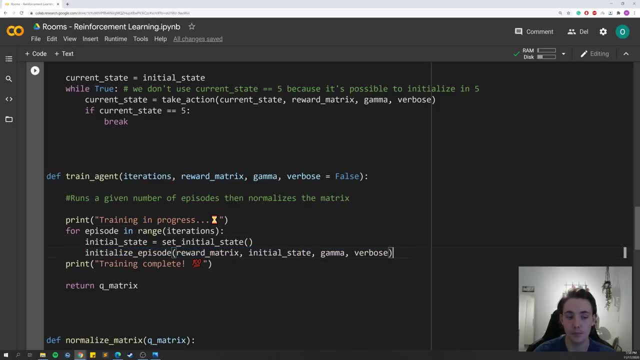 has reached goal five and then it will update the cue table while it's training. So we'll run this initial episode here. so we'll run like all the episodes- number of iterations, time- and then we just update the cue table and when we reach our end goal. 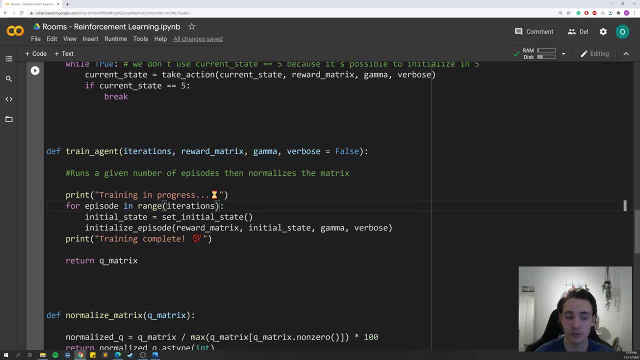 and then, after we've been through all the episodes, we will just print out like the training has completed and we have now updated our cue matrix and we'll try to estimate the reward matrix and then we can return that cue matrix or cue table and then we can. 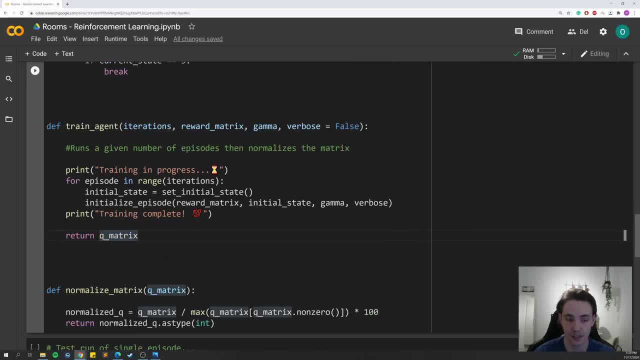 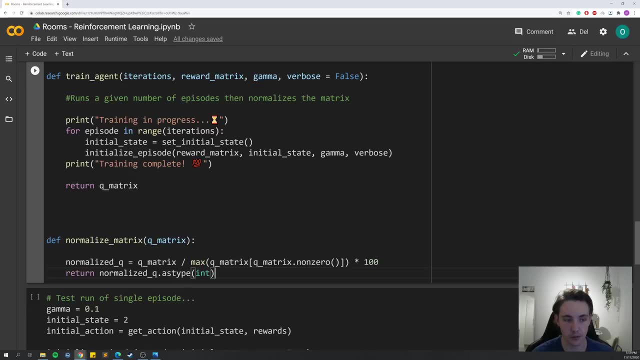 like display what we have learned by training this agent in the environment. Then we just have a function here to normalize our cue matrix. so it's a bit more intuitive to see the result of the training process. So we have control. control enter here, it will run the program. 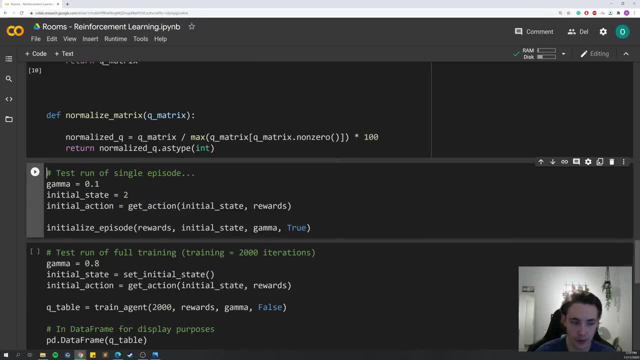 and we can go down here and test if it actually like works. So this case here we have this gamma factor here of 0.1 and the initial state here will be will be two. So in this case here we just chose, chose one, one initial state here. 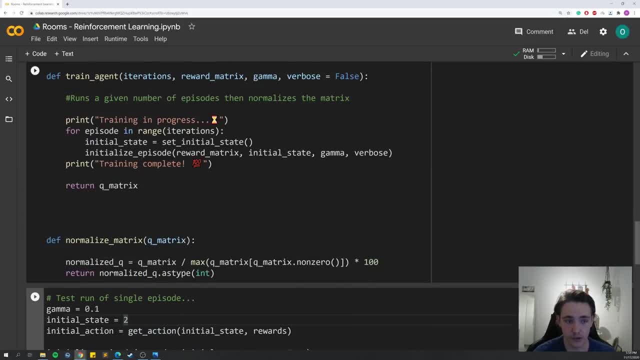 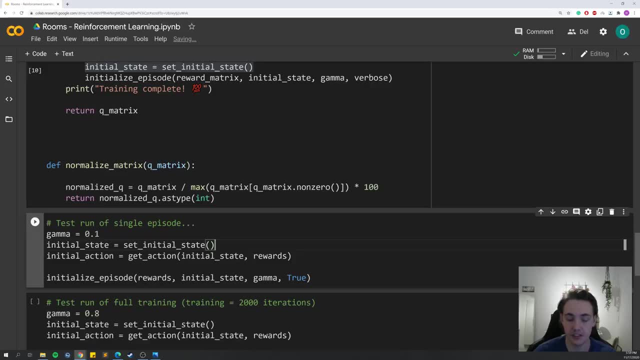 we can also have the set initial state, so it will like have a random initial state. we can also do that. so our initial state here will be equal to the random initial state here and then we pass that. pass that initial state to the get action function here. 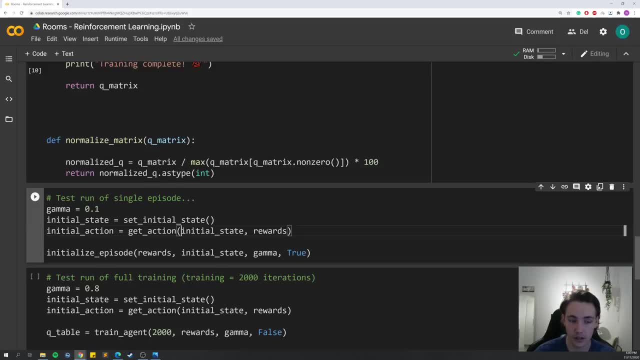 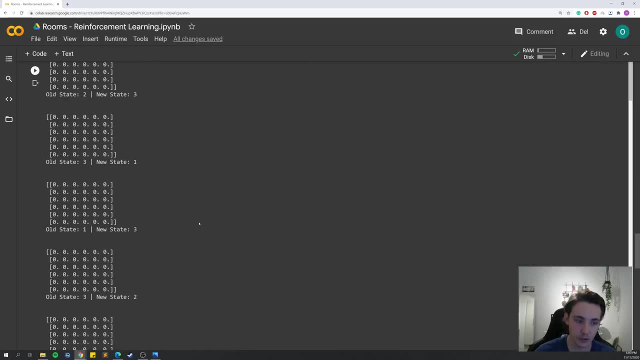 and we will get, then get an action, and then we can run our episodes here. so this is the case for one, one test, or like one episode that we're running over. so if I print this out here, we can see that we're we start at. we start at. 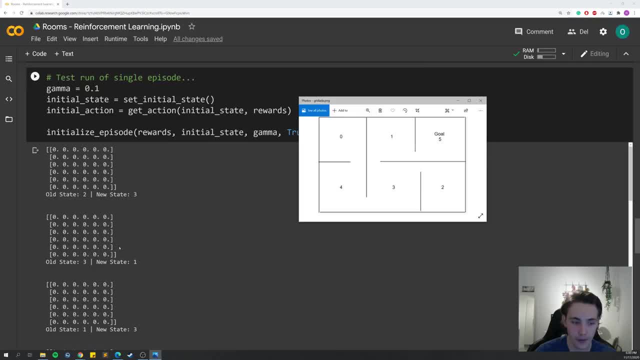 state two here and then we go to state three and then from state three here we go to state one and then from state one here down here or like we can also go from state three to two. but it didn't really like, we didn't really reach. 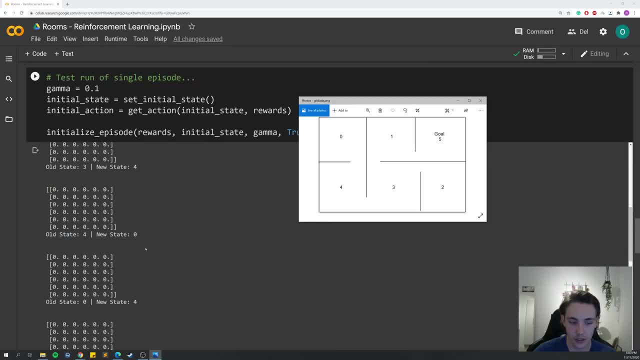 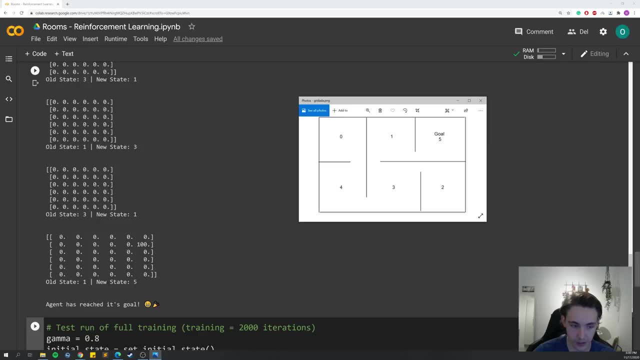 the goal here and then we can just keep on doing this until we reach our end goal down here. it ran over like a lot of different kind of episodes here, so now we have reached our end goal here and we can now update. now we have learned how to get from. 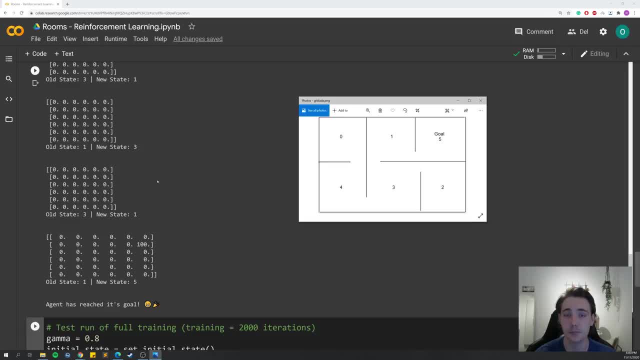 two here to five and it took a lot of different kind of we didn't know anything about the environment and we didn't have any rewards. that our agent has learned. so it didn't know anything about the environment and it had to learn all of it, but it has not reached. 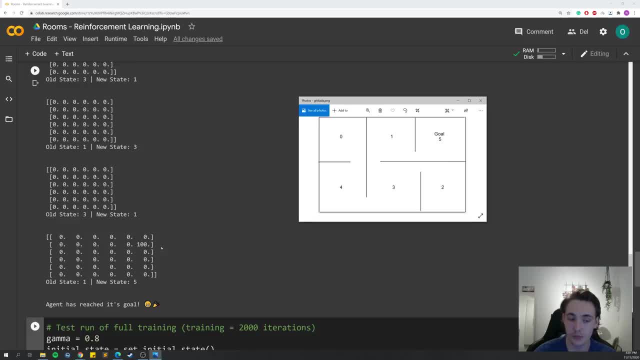 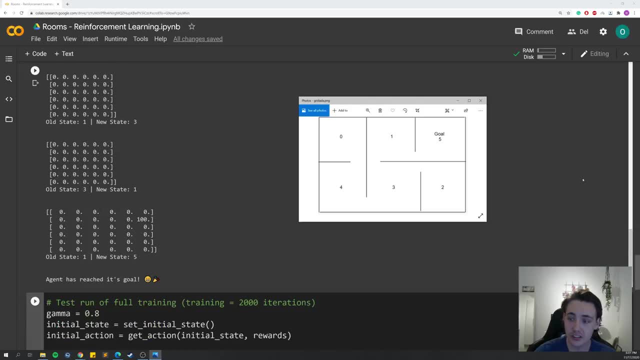 its end goal and we can see that that the reward, or like the queue function here or queue table here, is updated with this hundred here, because we got to get a reward of hundred when we restart in goal. so this is just an example of how we can run. 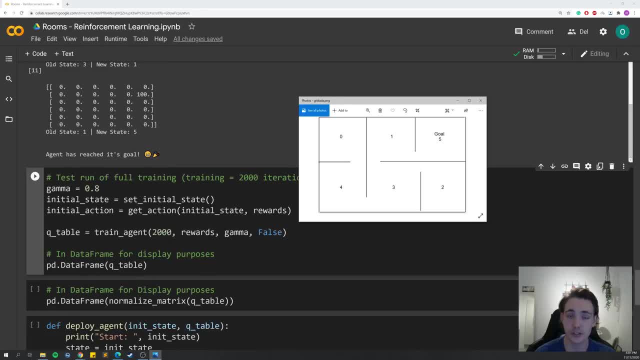 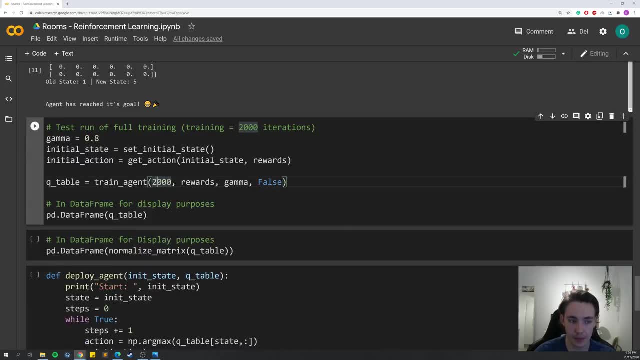 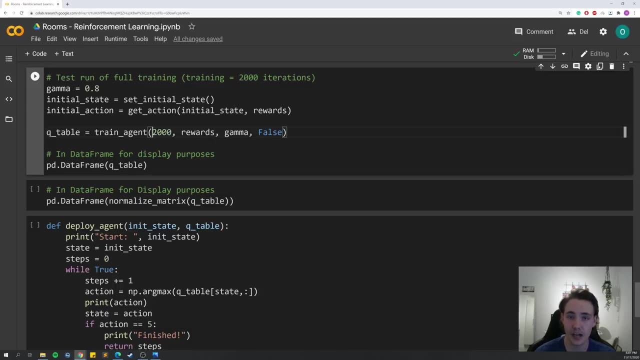 one episode of these episodes here to try to estimate the reward, the reward matrix, with our queue table. so to train our agent down here, we have this gamma factor here again and initial state, as we just did, and then we are going to run this process here for two thousand. 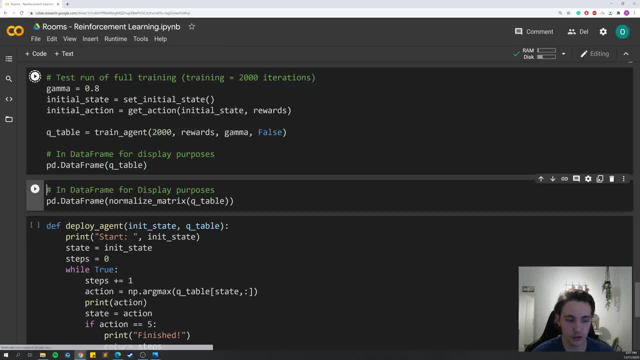 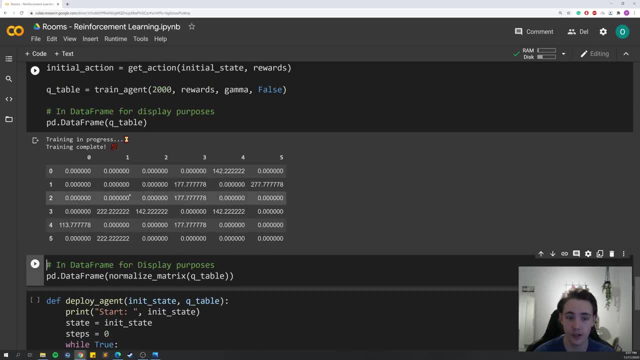 of times and then train our agent for two thousand episodes. and if you hit control, enter here. it will now train the agent in the environment and then it will print out the queue table here that we have learned from the agent. so these are like the values that we can take. 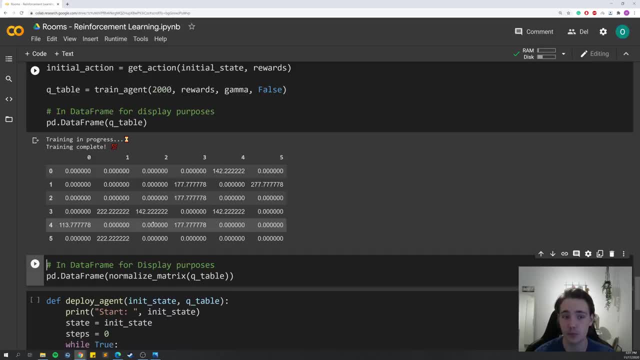 when we are going to apply or like deploy our agent in the environment and we are trying to get the shortest path and to the end goal which will return the maximum reward. so if you just wanted, like, we can just print it out here in the data frame. 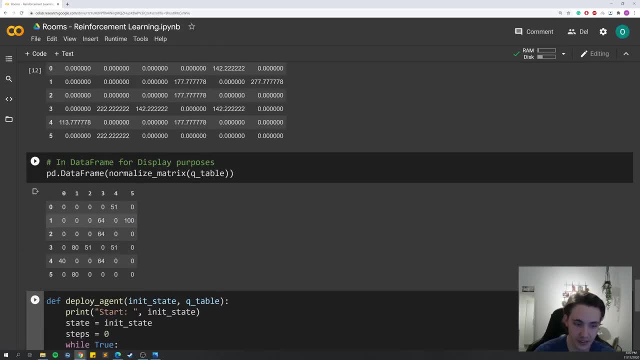 here when we have normalized this as well. so we can see that if we are in room one and we take, we can either take this action here or this action. but if we take the action five here, we will reach the end goal. and when we are trying, 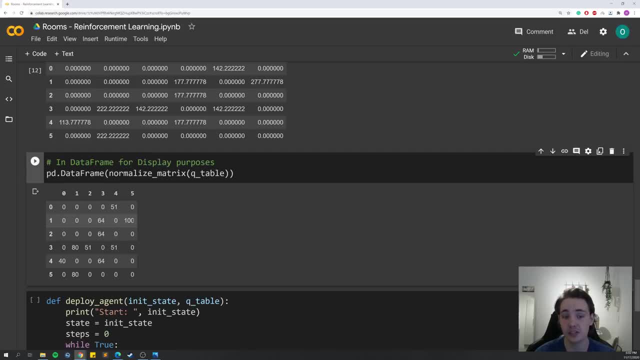 to apply or like deploy our agent with this queue table that we have learned, then it will always take the maximum value of these queue values here that it has learned for some given state. so it will always take the maximum reward that it is yielding here. so if we want, 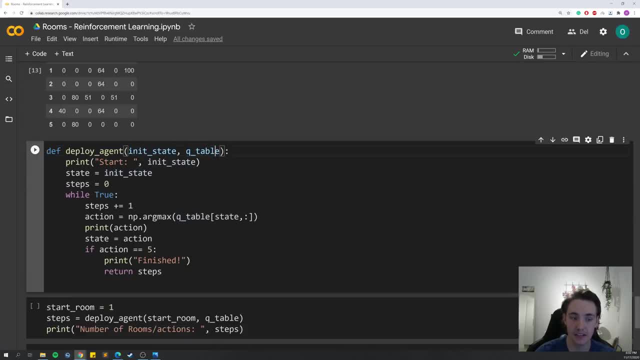 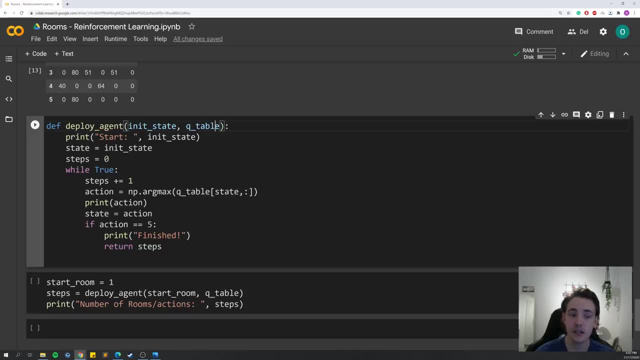 to deploy our agent here. it takes an initial state and then the queue table that it has learned and then we just set up this while loop here that runs through like as I just talked about: it will take the action with the highest, with the highest reward or like the maximum. 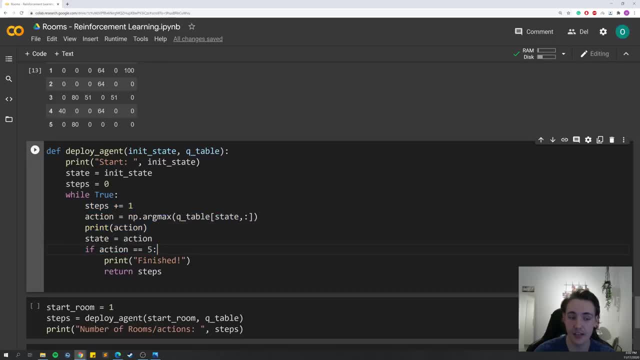 queue value in the queue table. so this is what this while loop here does, and then if the action is equal to five, then we print out it is finished and we return the number of steps that it took to reach the end goal from the initial state that we were in. 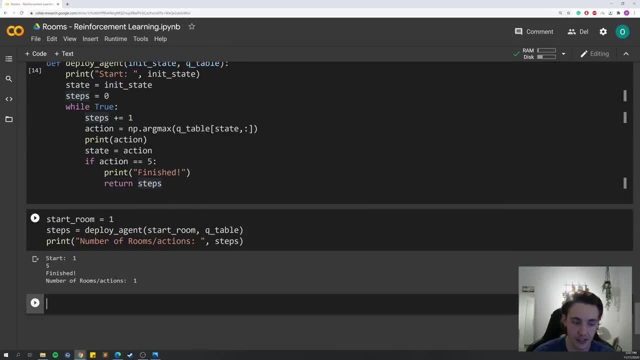 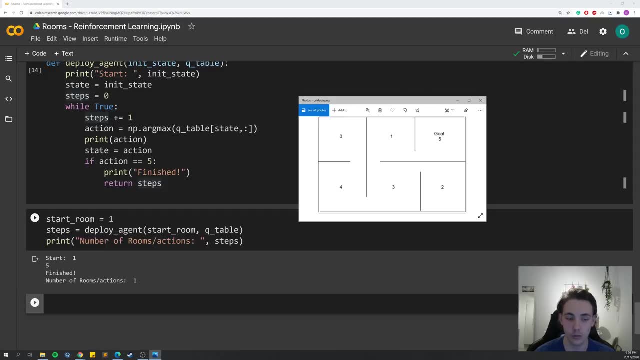 so we have control into here and if we go down here and deploy our agent, then we can see that if we start in room one here and the number of rooms in actions it took was only one, so if we try to initialize it over here in room zero, 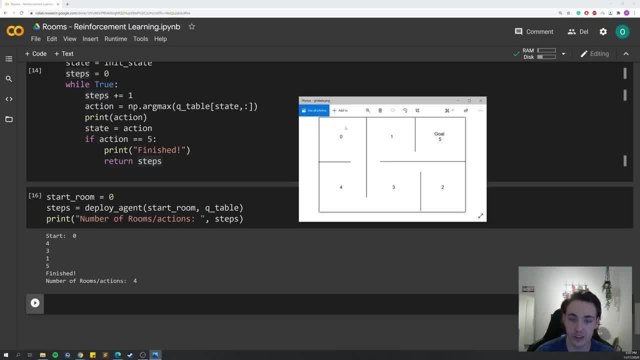 for example, and hit control into here again, we can see that it now takes four actions. so we'll go from room zero here and it can only go to room four. so we'll go to room four here and then to room three. but now it can. it can both. 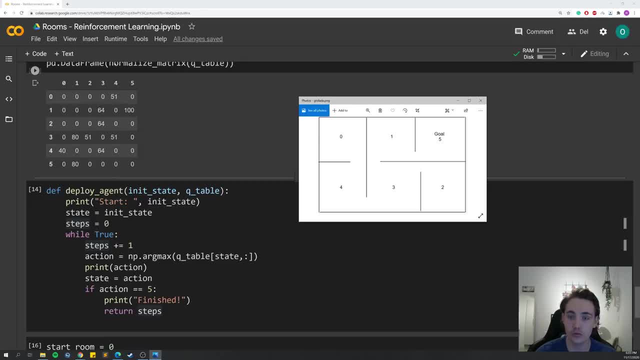 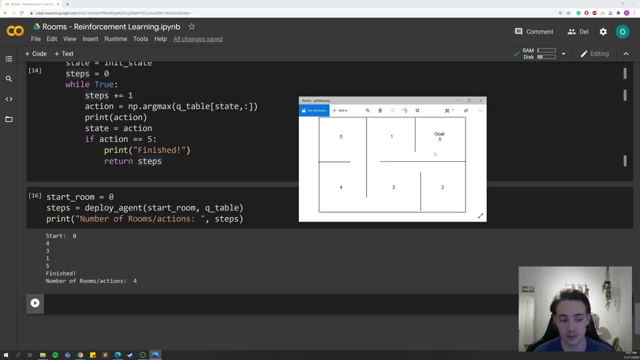 go to room two and one, but it has learned that we will go to room one because this is the maximum value 80 here. it will now go to room one and then from room one it will go to the end goal here, which is five, and we have now. 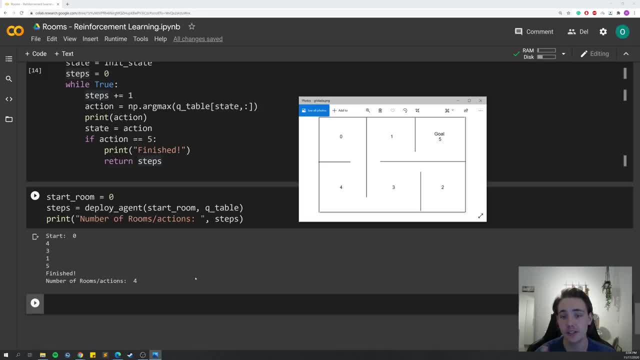 gone from from this room here to room five here by only taking four actions in the environment. so we can see that our agent has learned how to get from one room to the end state by just learning in the environment, from, from operating in the environment and apply.